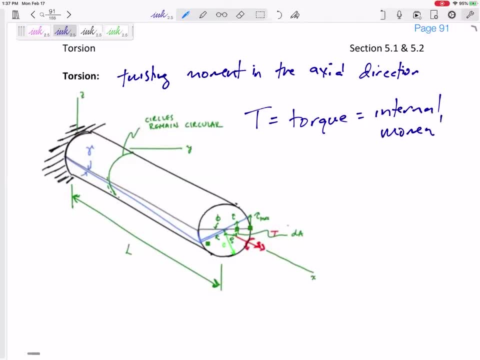 torsion, So we're going to call it T. It is a torque and it's an internal torsion. T is a moment about the axial direction. All right, it's what you think, right, Torque is a twisting moment T And, if you want, last year and in years past I've tried to derive this. 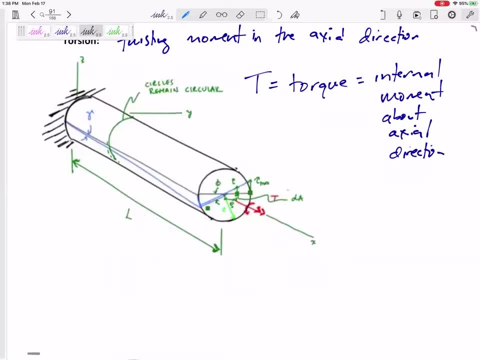 Let me take a look at it. draw one chickens, And then we're going to draw a little bit moreметid. you too? Ok, Let's do it again. So if you want to please pull it from structure, free this figure and the next figure, if you want the derivation, structural free does a lot better. 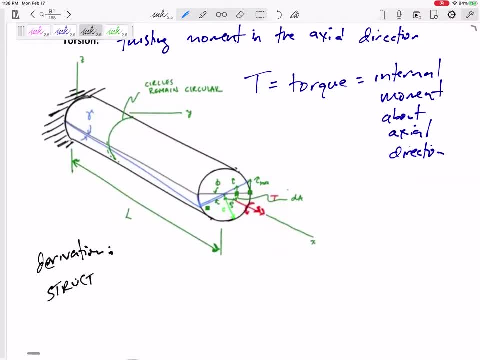 than I do, And you really should look up structure free on Youtube. anyway, A torque causes a stress calculated, yet All right. a torque causes a stress, The stress is. so you can. let's say this was one beam that was being twisted. Let's say this was one beam that was being twisted. 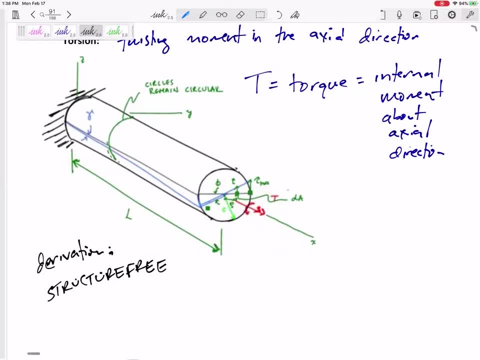 I had a torque on it. What type of stress would this face feel from this one if it was being stressed? What type of internal force, internal stress would it feel? Just kind of put your hand right here, It would feel a sheer stress. right, It would feel a sheer stress. All right, it would. 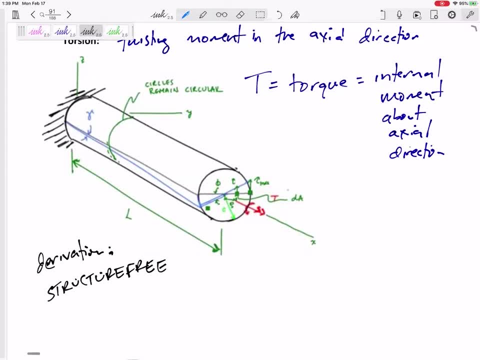 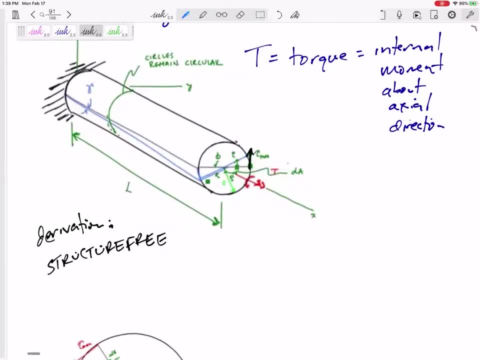 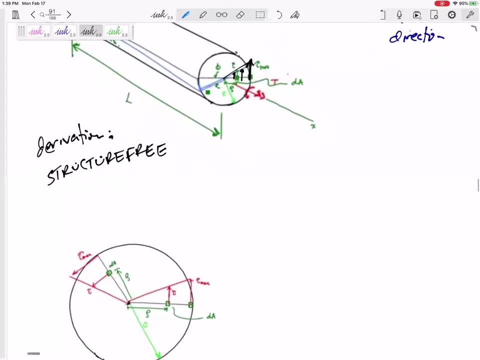 feel a sheer stress. I don't know if you can see this right here. It would feel a sheer stress that looks kind of like this: if we're right on the edge, As we get closer to the center it would get smaller and smaller. That's what these two diagrams show. It would feel a sheer. 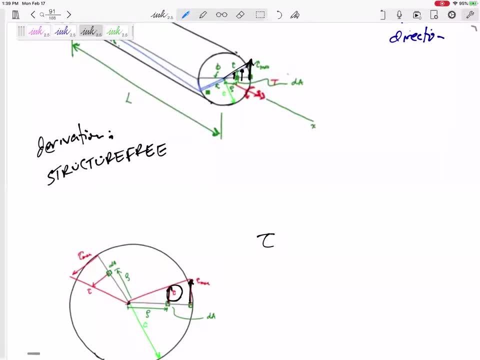 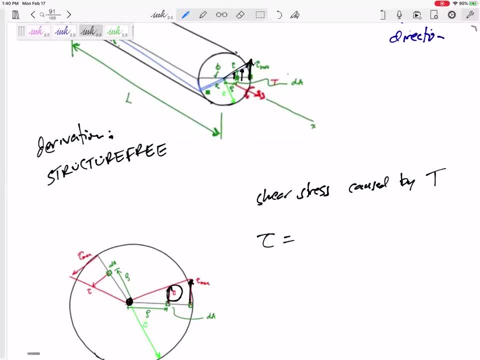 A little square on this face. If you were on the outside edge, you would be getting sheared more than if you're close to the middle. close to the middle, If you were at the middle, you would not feel any sheer stress due to this internal torque T. 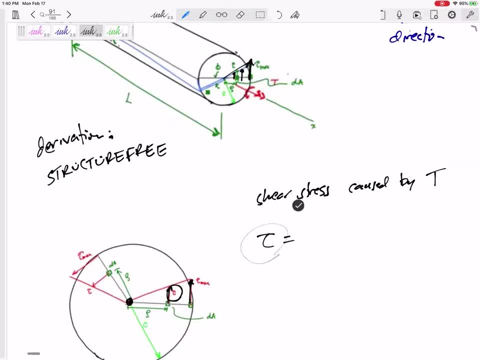 So what would the magnitude of this sheer stress be? we could kind of guess, we could think about a few things. uh, the larger the t, the larger the shear stress you would feel. uh, and then this row is how far you are away from the center of the cross section. 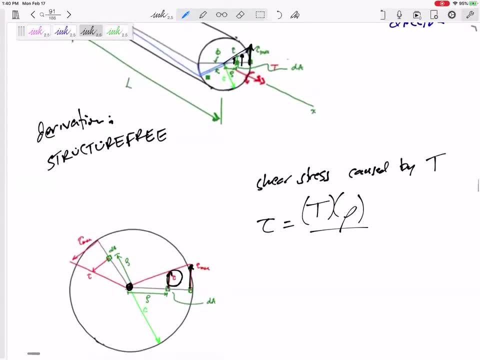 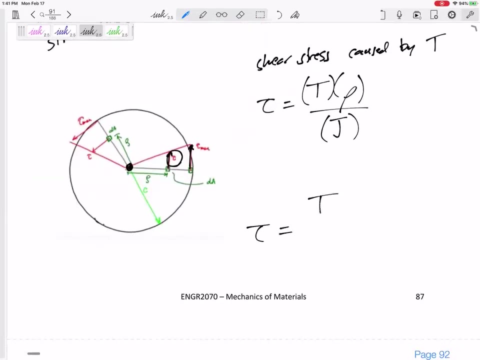 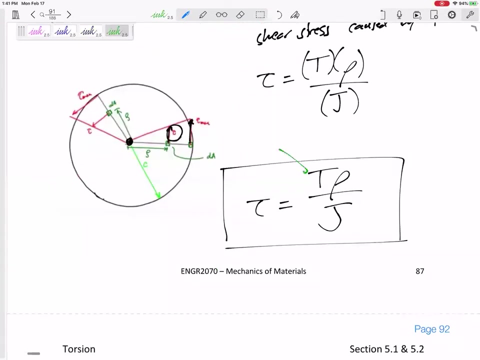 and then we're going to divide it by j. j is the polar moment of inertia. so let me rewrite this real big t. row over j, the shear stress caused by torque. is t. row over j. t is the internal torque, the internal moment in the axial direction. row is the distance. 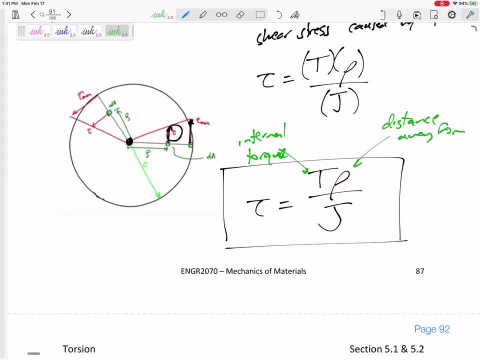 away, away, away from the center, really the center of gravity, the center of the cross section, and j is the polar moment of inertia. um, it is a measure of how much area is away from the center of your. um, the center of your am the renting are celebrating the size of your cross section. um, you know, mass moment of inertia. 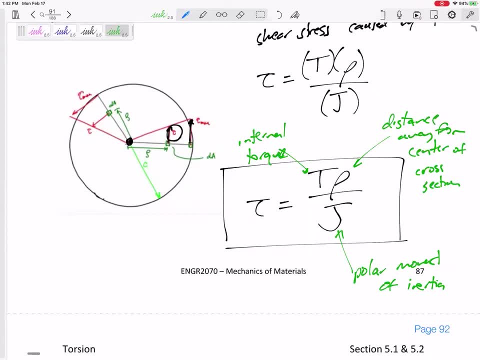 is measured how much mass is away from your rotation area. moments measures measure how much area a pole moment inertia is a measure of how much area is out from the center and didn't have to think about that. far out radiolally is from the center existing power that you're in 우. 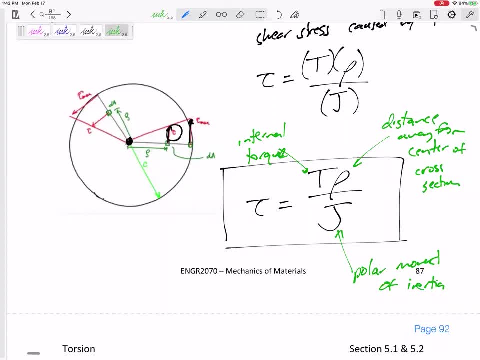 polar momentum. inertia is measures the it's resistance to twisting, its resistance to twisting. and next paper is the version that we use as our per woods in our common sense, such as is the equator, its axis, wasур to prectawa, that we're going to saddering an Queolla're trying- not i mean 99%- in order if there is a error. if you got that, sa perché? um, there's gonna be more input from us conversation. we're gonna get some. So base up on ReadOn…. 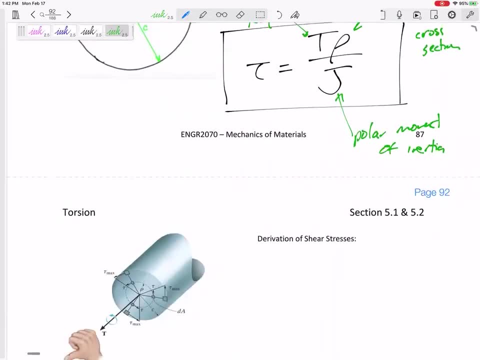 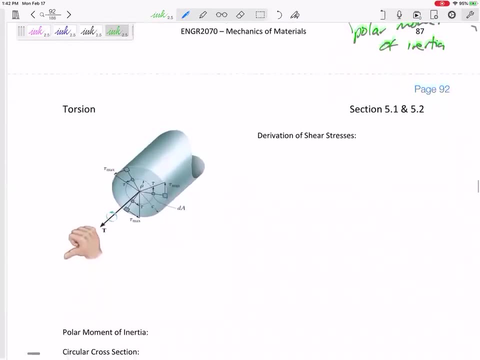 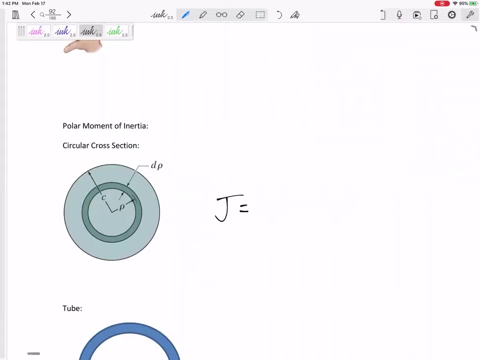 point, last note. there's one major thing that I want to wrap up: What's the most significant factor in the paper? here page, Next page, We could also derive this, But next page the polar moment, inertia. and this is on your formula sheet. You still have that formula sheet. Technically it's the 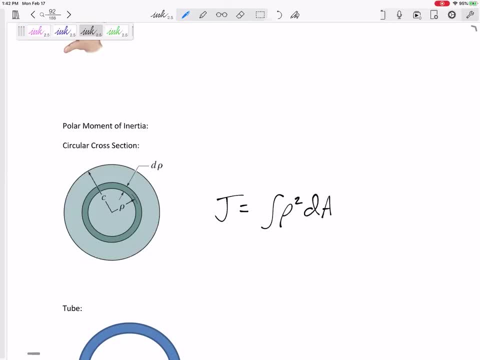 integral of rho, squared dA, but for a solid circular cross-section, one-half pi. The book might say c to the fourth. It's just the outer radius to the fourth. I'm going to put r to the fourth. It's one-half pi. r to the fourth. Be careful and don't mix this up. Area is one-fourth. 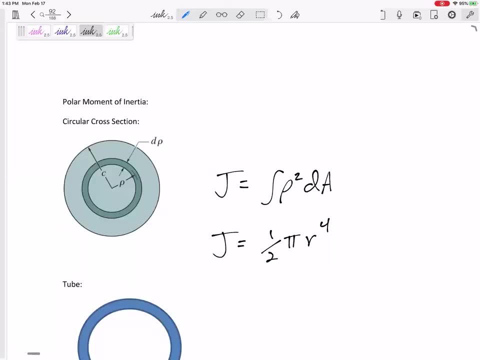 I r Square right, Or pi diameter squared, Or pi r squared. I'm messing it up now, But don't mess up that one. It's one-half pi radius to the fourth. One-half pi radius to the fourth. Make 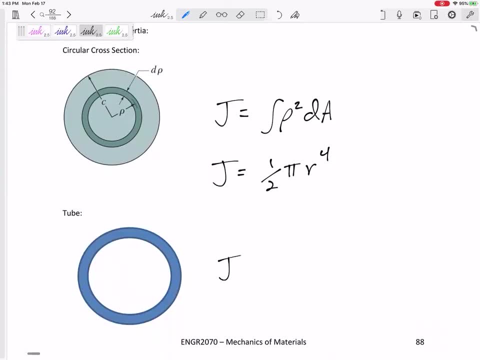 sure I give that to you. Yes, For a tube. this is one-half pi. You probably could have guessed this: r outer to the fourth minus r inner to the fourth. The book probably says c outer to the fourth minus c inner to the fourth, But c is just the outer radius. 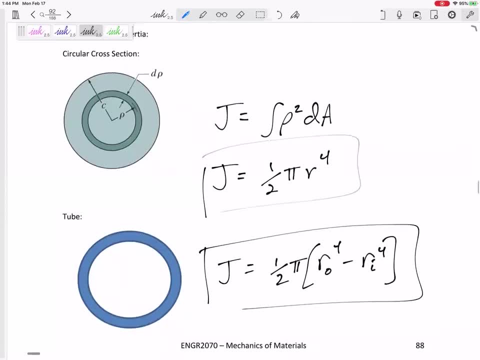 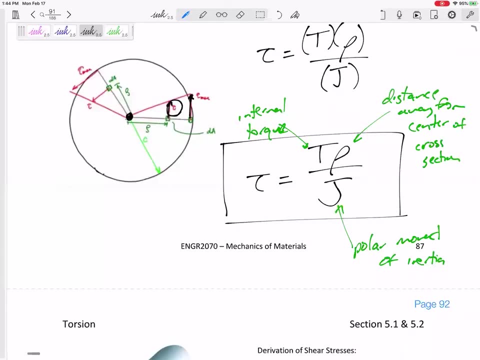 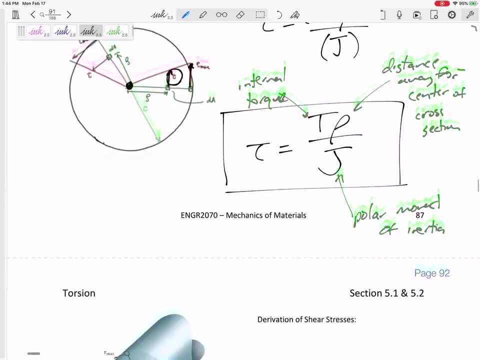 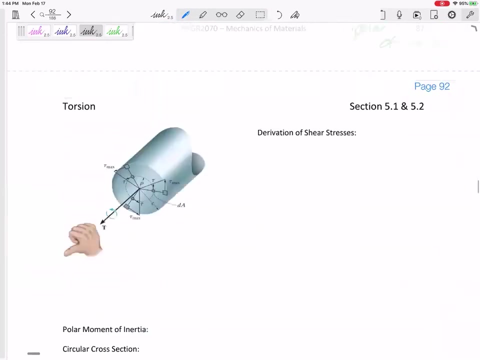 Okay, Let's just simplify it down to that: The stress, the shear stress caused by a torque, tr over j And I might even say r over j, But this is how far you are away over j, And the j is one-half pi? r to the fourth. Now, what direction is this? 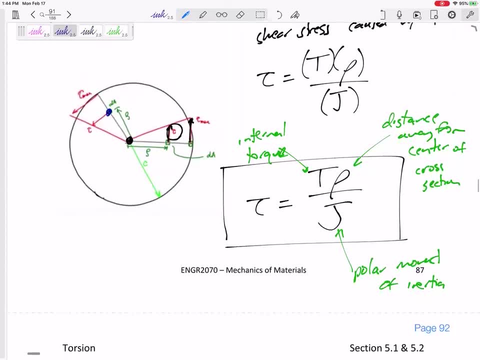 torque. Well, it depends. If you're right here, the direction would be right here. If I'm right here, the direction of that stress would be right here. The direction of that stress while y'all are in my dynamics class. the direction is perpendicular.